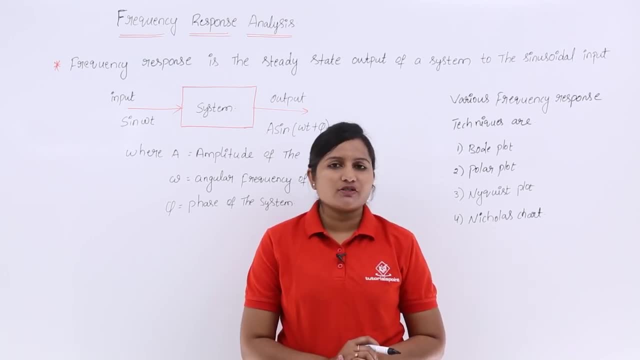 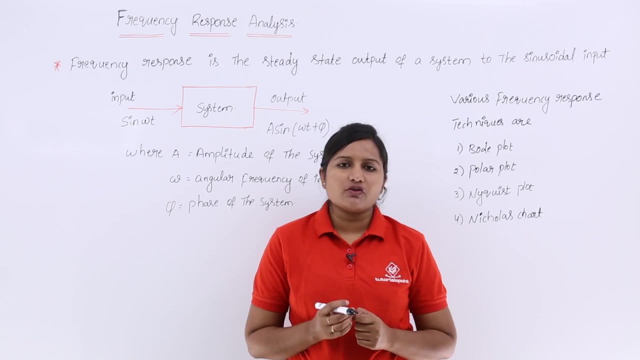 In this video we are going to discuss frequency response analysis. First of all, frequency response analysis means this is the response of the system. So for sinusoidal input, that means the definition for frequency response is: this is the steady state response of an LTI system. 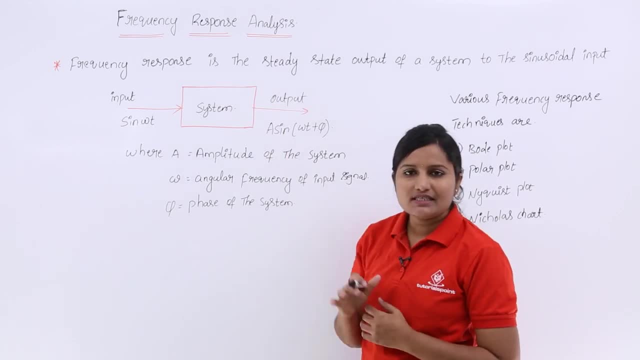 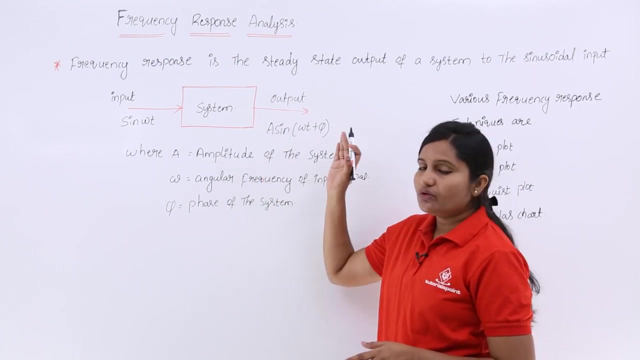 for sinusoidal input. For example, if this is your LTI system, if you, given any sinusoidal nature of input, If you are exciting your LTI system with sinusoidal signal like sin, omega t, cos, omega t, like that, So then you will get the same signal out at the output. So that means 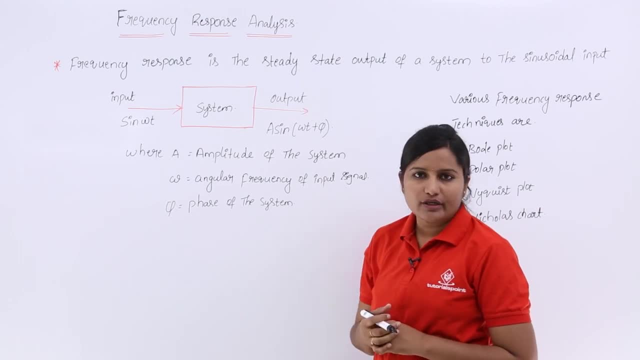 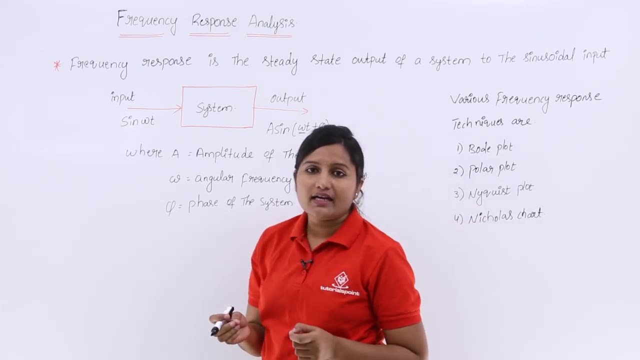 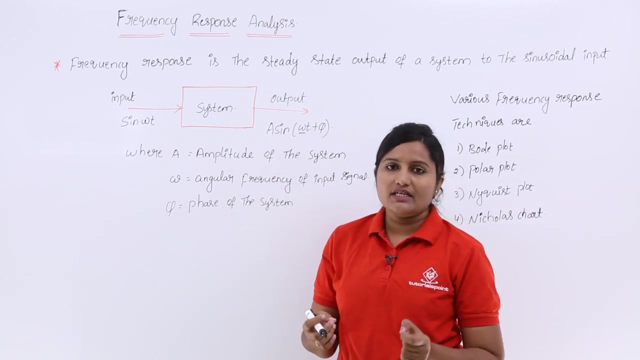 so you can observe, the amplitude and phase are going to vary, but the frequency is not going to vary. When The frequency is not going to vary means you are getting the same signal at the output with increased or decreased amplitude. that increase or decrease in amplitude and change in phase. 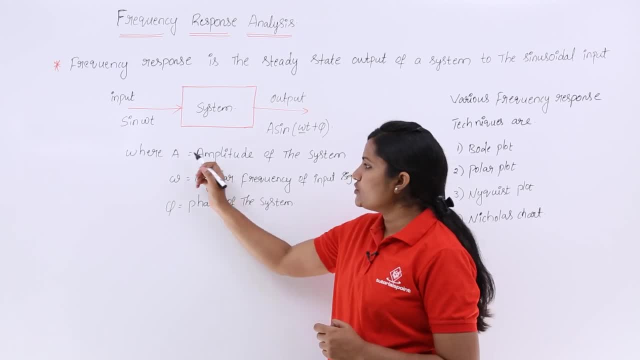 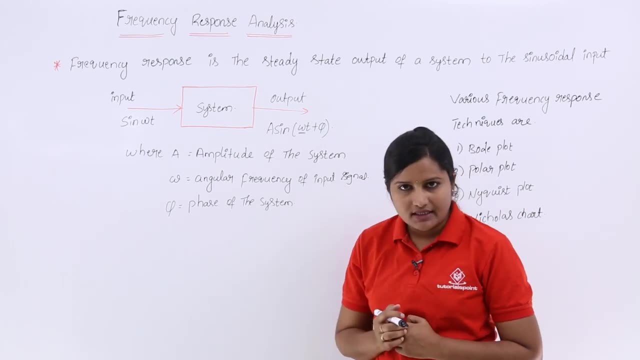 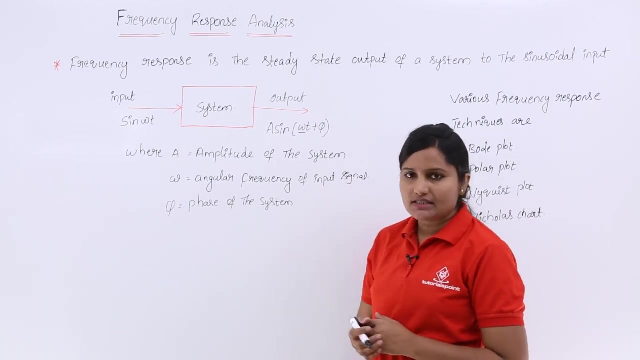 is due to the system characteristics. So coming to A, where A is the amplitude of the system and omega is the angular frequency of the input signal, same will be maintained at output also. and coming to phi, So phi is the phase of the system. because of that system, how much phase. 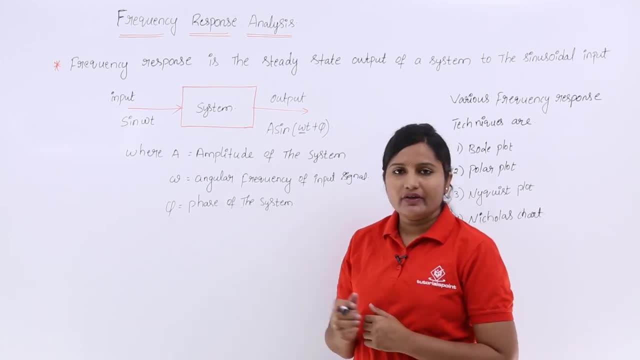 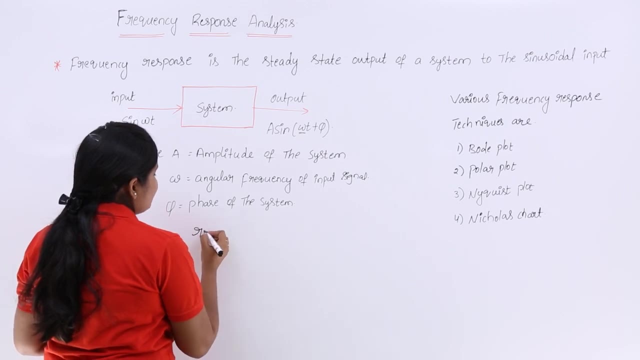 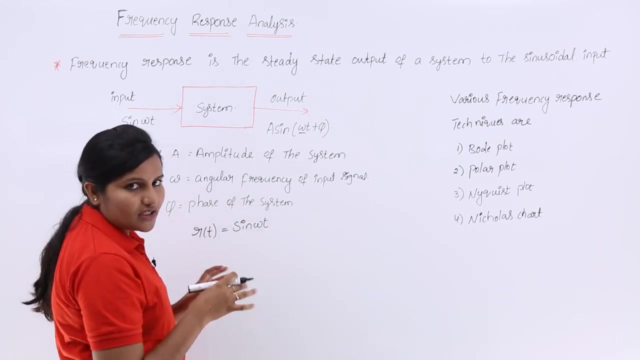 this input signal is taking. So that much phase we will indicate here. So, for example, if you are considering sin omega t as input for your control system, that means R of t is equivalent to sin omega t or sin omega naught. in some textbooks you can see omega naught t, omega a t. 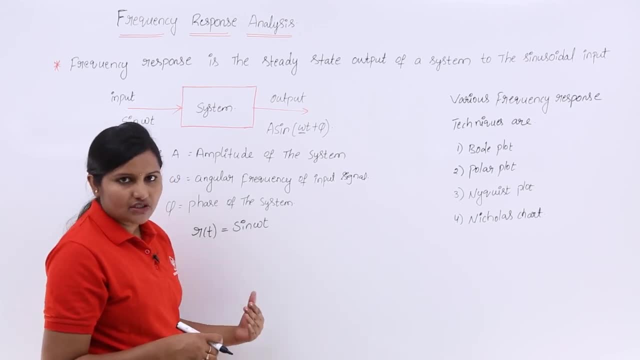 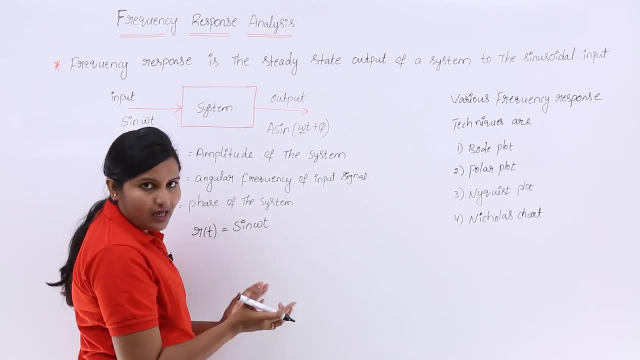 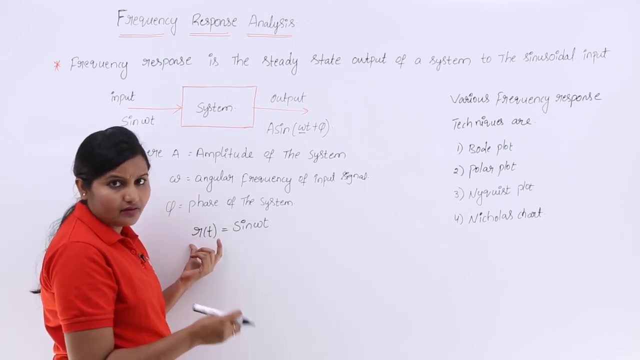 like that, So you can consider as your wish. the naming of the frequency is like your wish. So here I am considering like R of t is equivalent. R of t means, you know, in control systems R of t is generally represents the reference input. So here R of t is equivalent to sin omega t. I consider like this: 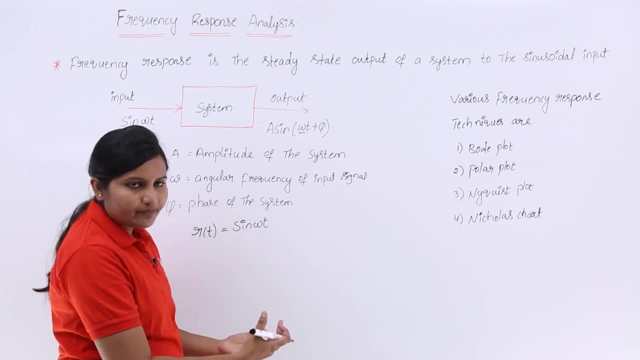 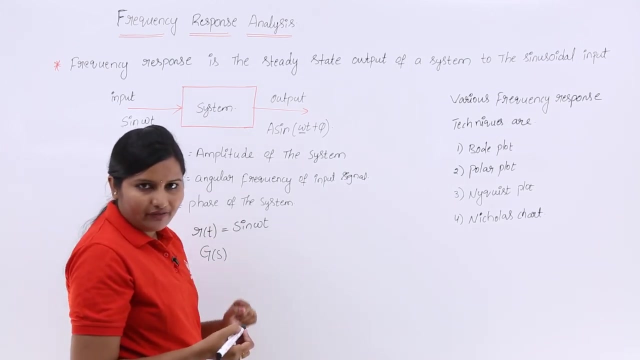 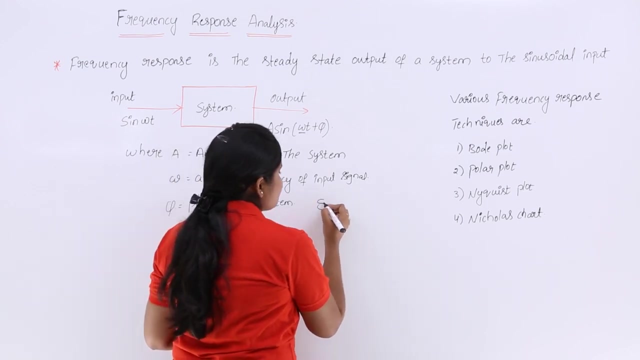 So, after considering our signal, what we are doing? So we are giving the signal to a LTI system. So now I am considering that LTI system open loop transfer function as g of s. So here as we are giving the input signal as sinusoidal signal or sin omega t, definitely you can substitute s is 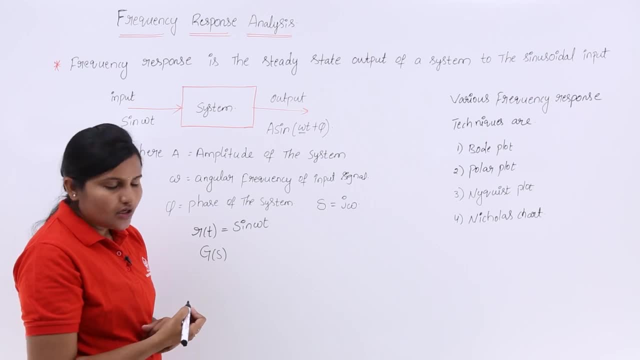 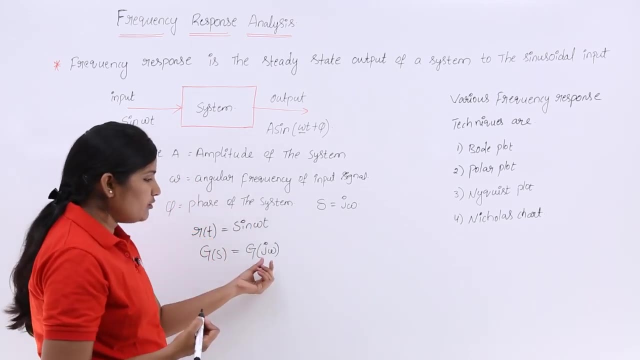 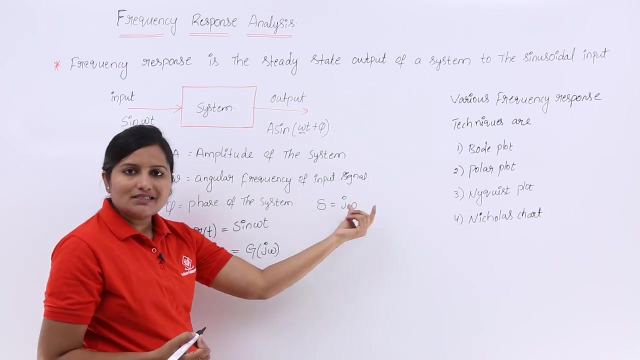 equivalent to j omega in your transfer function. So now onwards, I am going to substitute. So in s place I am going to substitute j omega. why? Because our input is a sinusoidal signal, So s will become j omega, So that frequency 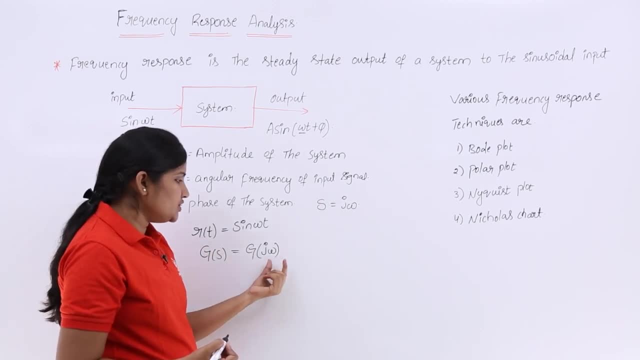 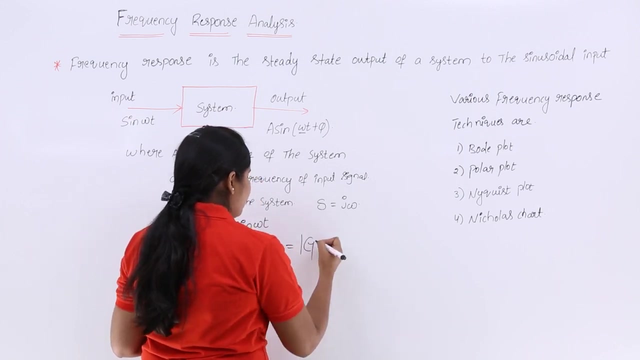 factor you will get here. So g of s is equivalent to g g into g of j omega. So here, in place of s, I am going to substitute j omega. and now we can represent this transfer function like this: in terms of magnitude and phase g of j omega. this is magnitude and in terms 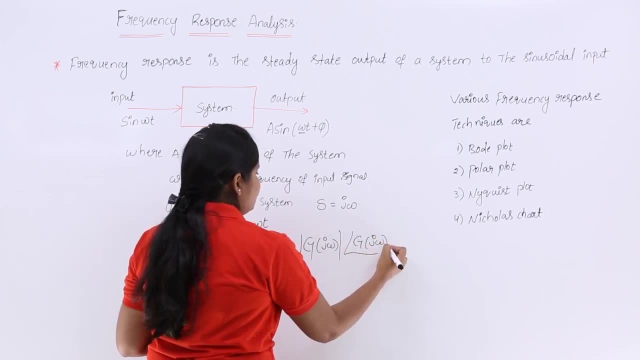 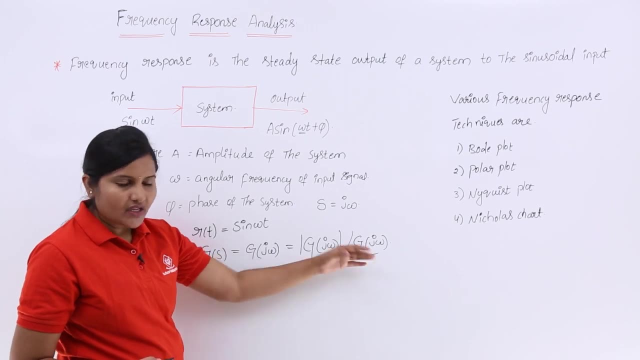 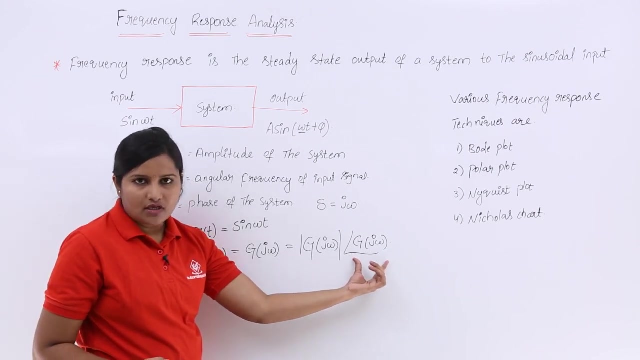 of phase angle. So this will be your transfer function. So now you can represent your transfer function like this: this is called as magnitude spectrum, this is called as phase spectrum. So here this is magnitude and this is phase spectrum. so here this will represents the 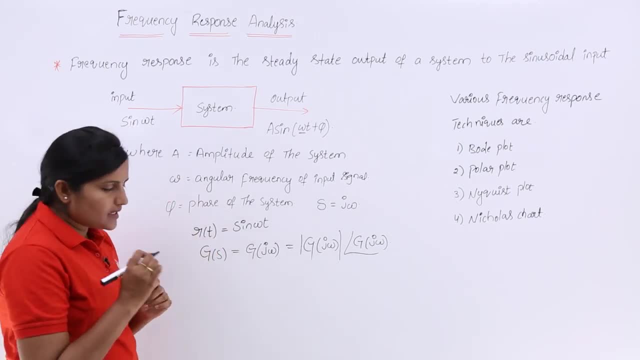 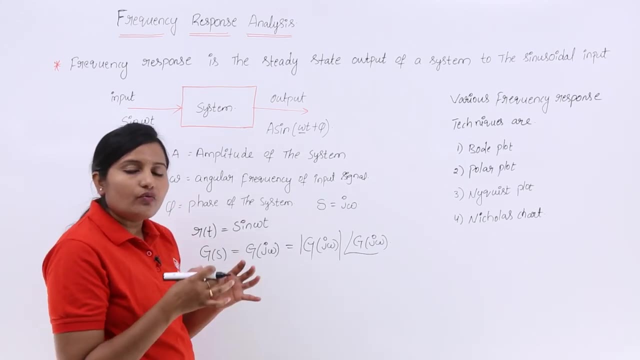 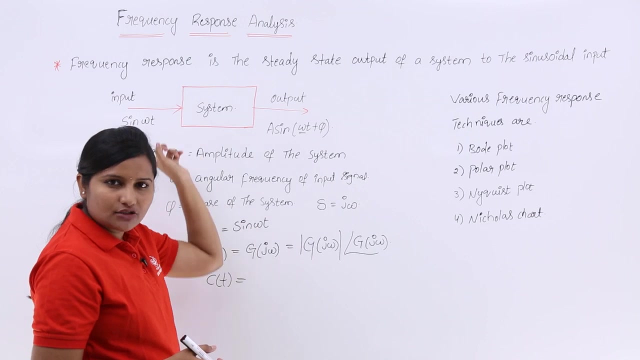 amplitude and this will represents the phase. If you want C of t, that means output signal. how will get output signal? So, first of all, what is going to done? for output signal means if you given this signal to this system, according to the characteristics of the system, the amplitude is going to vary and phase is going to vary. 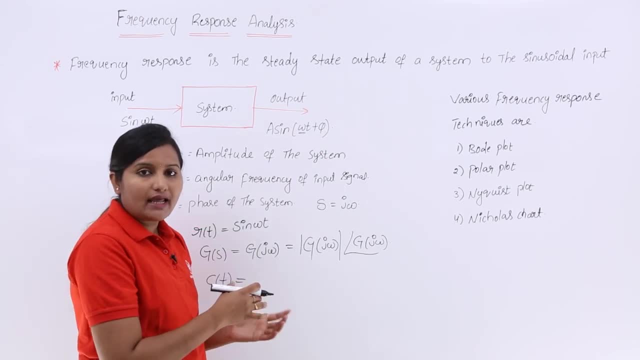 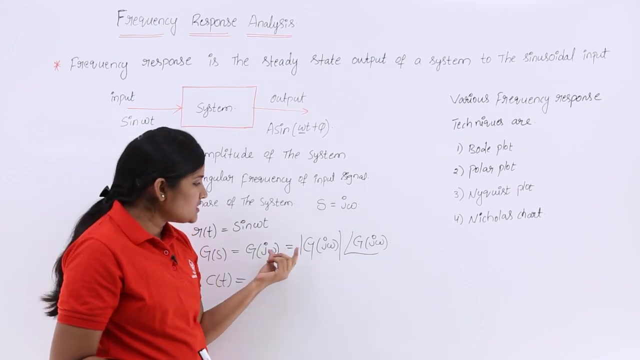 So how we can give that amplitude, how we can write that amplitude means, in terms of this magnitude spectrum, we need to write that amplitude. and coming to this phi, So this phase angle, we need to consider why? because g of j, omega is the transfer function of the system. So, according to, 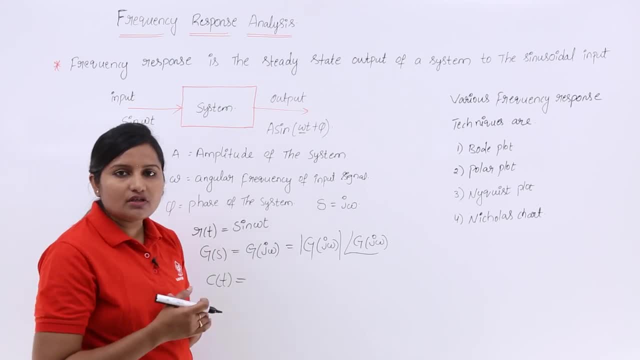 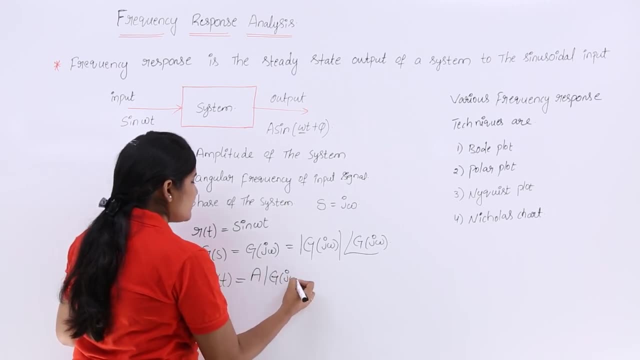 that transfer function, so the output signal is going to come. So here C of t is equivalent to a into more or less of g of j, omega. I am considering like this: So that means so in terms of multiple of magnitude spectrum, or so in terms of multiple of magnitude spectrum. 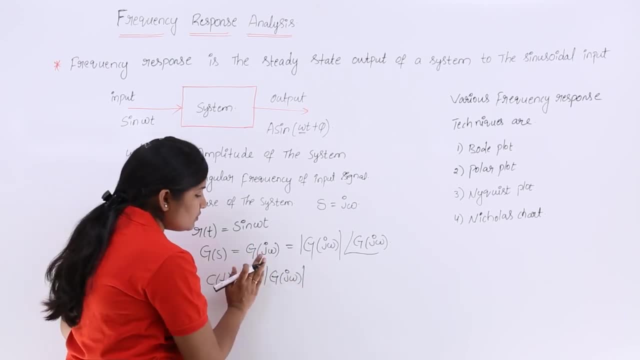 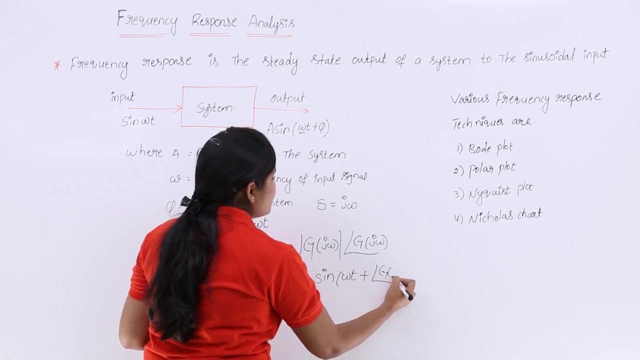 or multiples of magnitude spectrum. that means so, like this also, you can consider after writing whole thing. I will explain you. C of t is equivalent to a into g of j, omega into sin, omega t in place of phi. I can write this phase spectrum So: 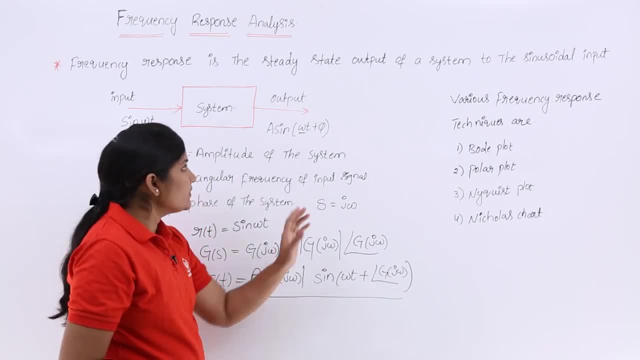 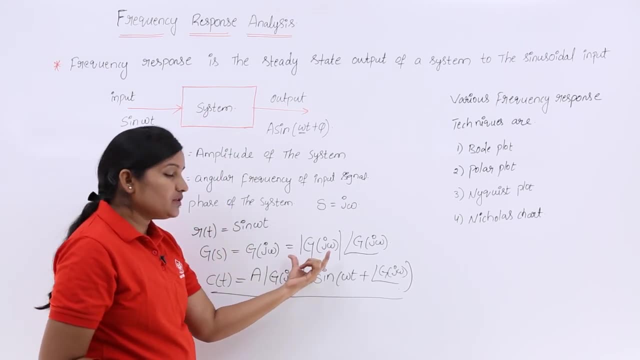 this is the output signal. so that means, if you observe, So this amplitude will vary according to the system transfer function. so that is why, So this output signal amplitude can be calculated by taking magnitude spectrum in multiplication. So you can see, this is: 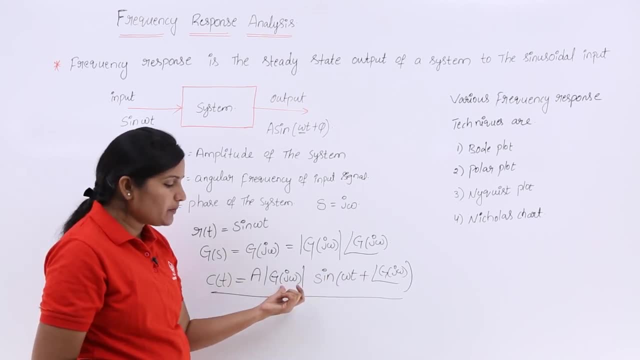 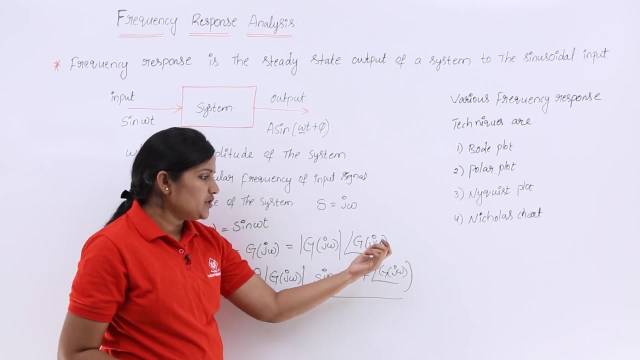 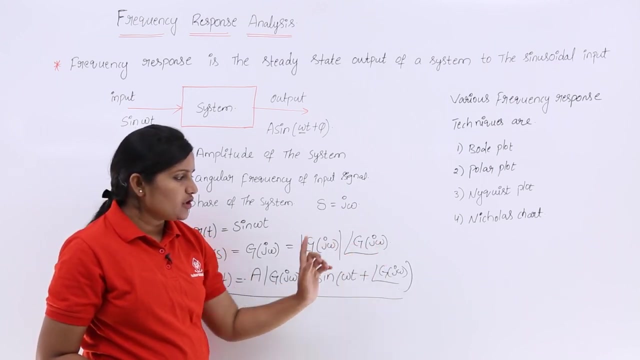 multiplied with magnitude spectrum. input signal is multiplied with magnitude spectrum or multiples of magnitude spectrum. And here, coming to the phase angle, you need to consider the phase of the system. So phase of the system is nothing, but so angle of g, of j, omega, this will be your output signal. 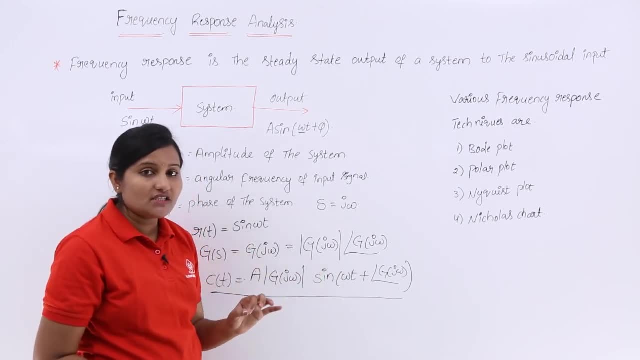 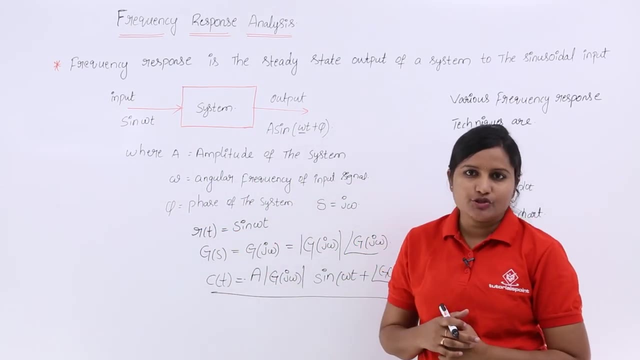 in this signal, omega is not going to vary. the frequency of this signal is not going to vary. that means you are getting the same signal with increased or decreased amplitude and change in phase. So this about a frequency response of the system. nothing but the steady state response of the system. that means this: this is the 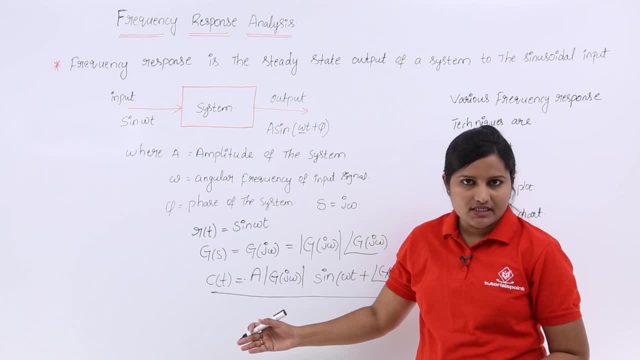 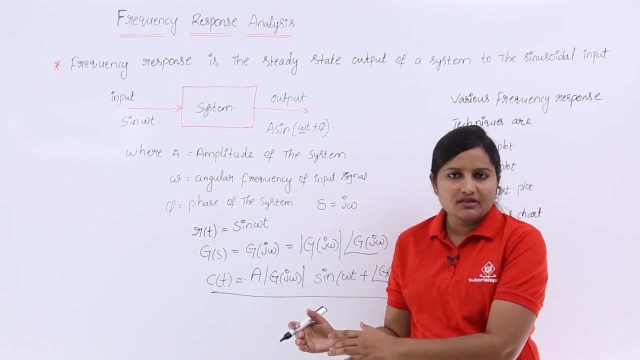 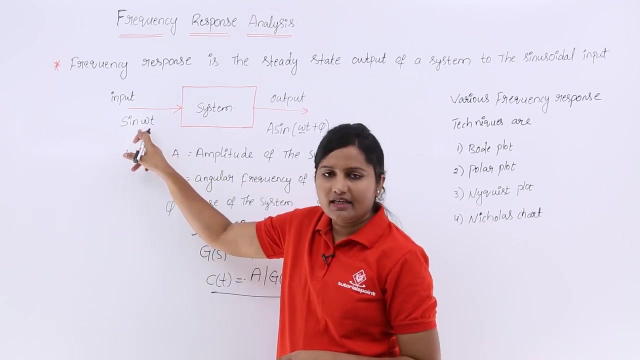 frequency response. Response is nothing but output of the system. frequency response means when you given a particular frequency, the response of the system is nothing but frequency response. Frequency is generally given in terms of sinusoidal signals. that is why I given sinusoidal sin omega t. So here this is the meaning: I given some frequency as input. 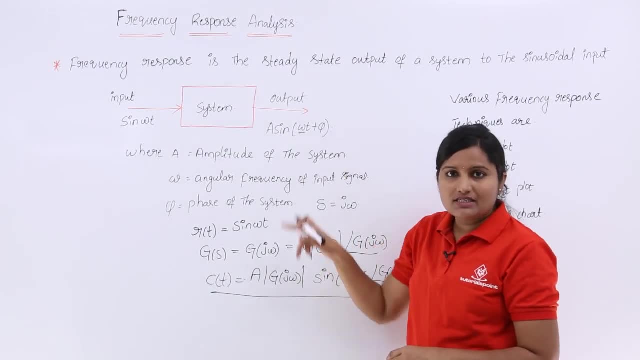 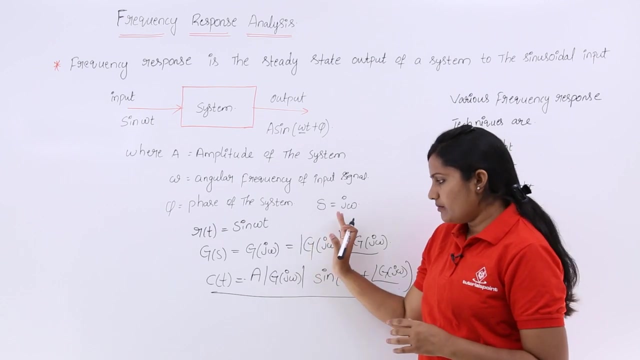 signal. So the response of the system for that frequency is called as frequency response of the system. Now c of t will be the frequency response of this particular system. How we are calculating that frequency response means So here just by multiplying our magnitude.